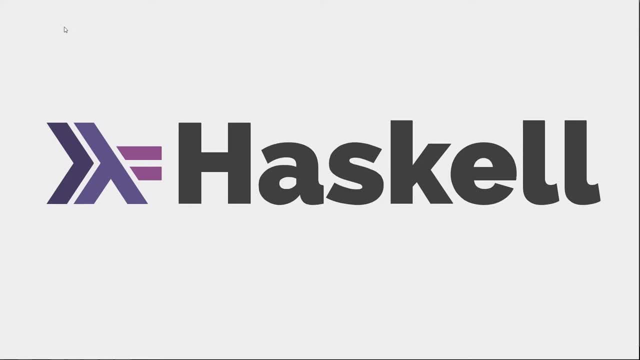 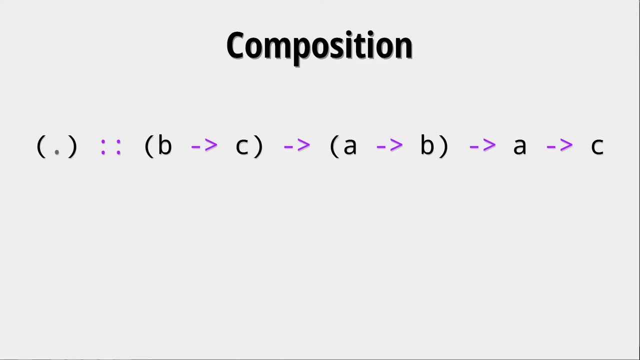 In this video we are going to look at function composition, a neat and elegant way in order to combine functions in Haskell. For this we will use this dot operator or composition operator. This dot operator takes two functions as arguments, and then a value, and gives us back a value. 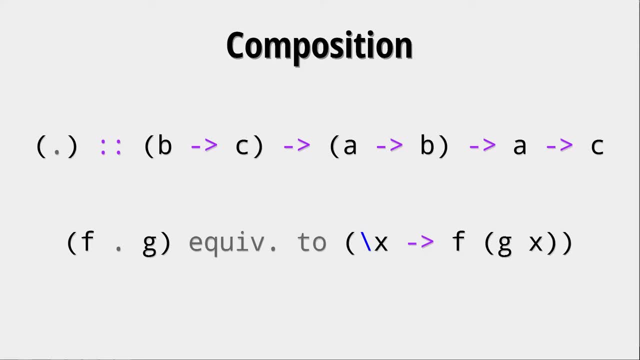 So when we have a term like f dot g, it is equivalent to the anonymous function where we have some free variable x and then first apply g to it and after that apply f to it. So what can this be used for? Well, for example, let's say you have an ascending sorting function. 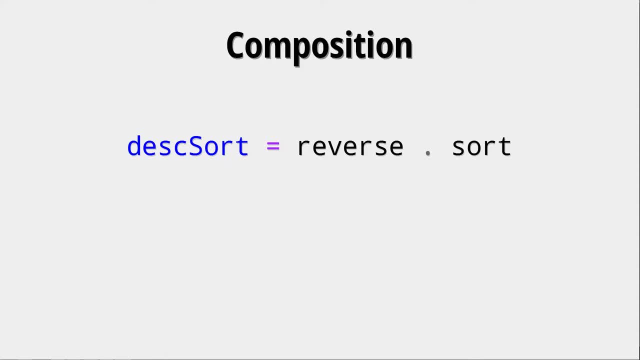 like sort, and you have a reversing function like reverse. you could construct a descending sorting function by doing this little composition. Now, why is that This true? well, those three definitions we have here are completely equivalent, and we can see, step by step, how you get to the last result. Well, if you use the equivalence, 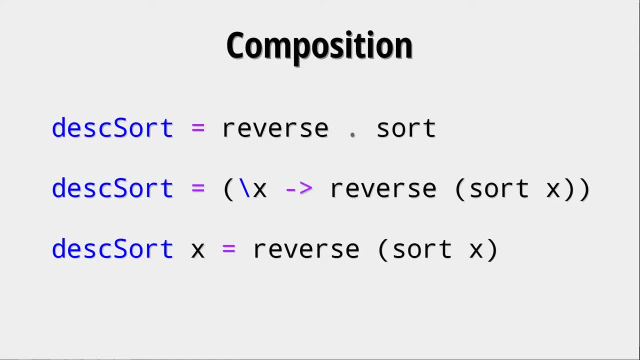 of this dot operator, you get this anonymous function definition. and if you now take the free variable x and just put it into the argument list of descending sort, we see why this is true. We can also see that we didn't need any arguments in the descending sorting function before, because 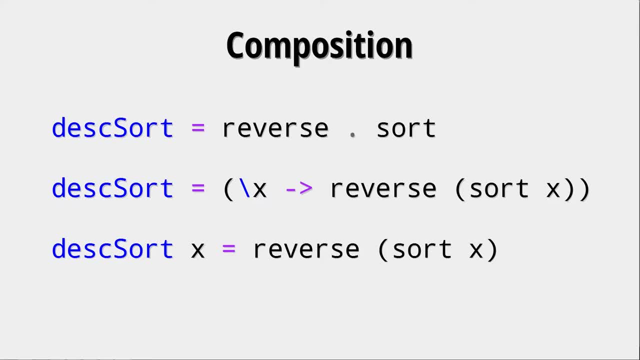 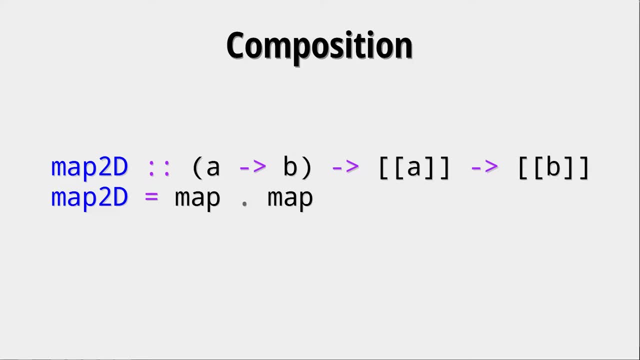 we get a function back that already needs one argument from the composition. A more practical example maybe would be a two-dimensional map. Now it's very important to see that this function that we give it still is only a to b and not, for example, n list of a's. 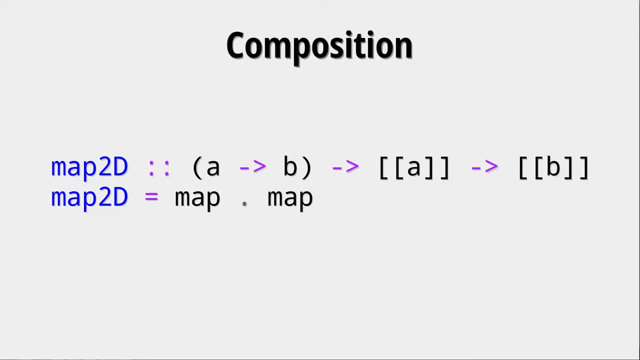 But this map2d now works on two-dimensional lists. By the way, doing this with multiple maps- so mapmapmap for n times- would create an n-dimensional map. So doing this with three maps would create a map 3d, for example. It's not that trivial to see why this is true, so let's go through. 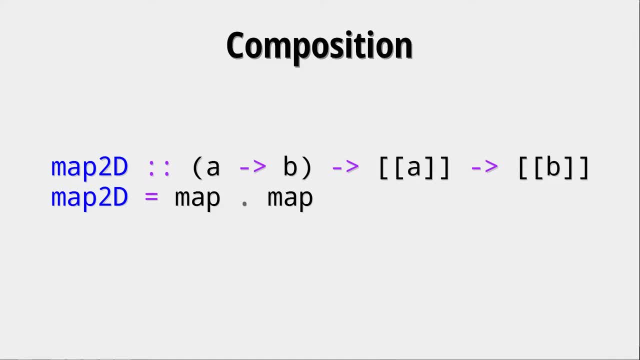 it step by step. All of these things that we've seen so far in this tutorial will help us to understand why this is true, So let's go through it step by step. All of these things will help us to understand why this is true, So let's go through it step by step. 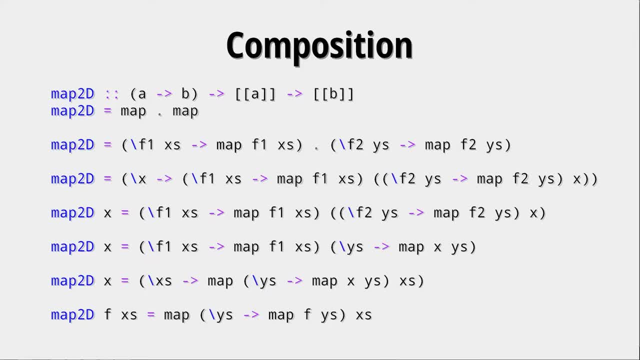 All of these definitions that we have here are equivalent, And in the last definition we should sort of see why this is true. but let's go through it again step by step. Well, if we have the term mapmap, we first replace the single maps with anonymous function. 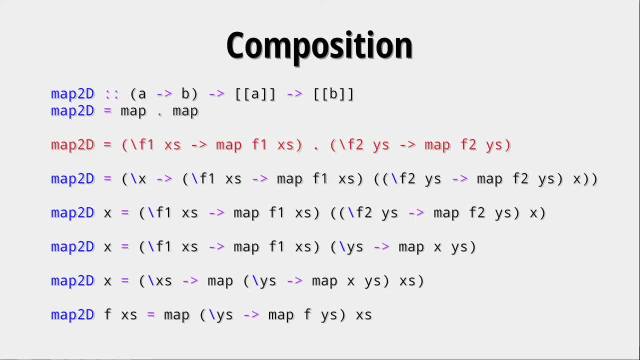 definitions, because a single map takes two arguments: It takes a function and it takes some list. So we have to write this explicitly here in order to see how those functions will combine. Okay, in the next step we do the equivalence of the dot operator and in the following step we take this free variable x. 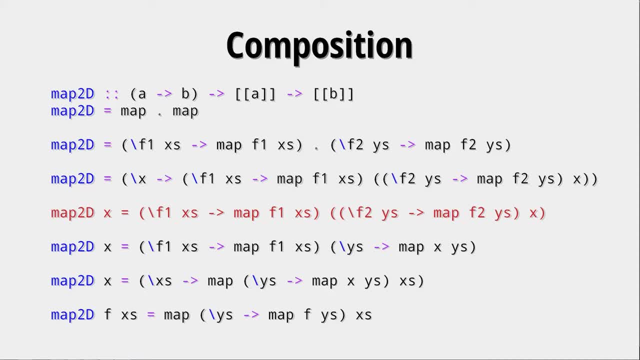 and put it into our argument. list of map2d. Now a more interesting thing is happening because the free variable x is applied to the anonymous function definition f2 ys to map f2 ys. so x would be the first argument of this function, which is f2. so we replace f2 by x and of course, 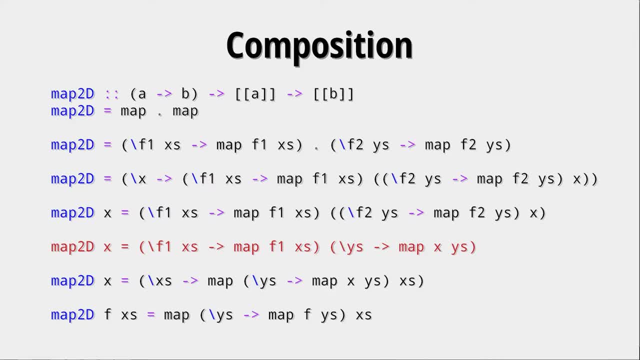 f2 is now missing from the argument list of this anonymous function. Now, in the next step, another interesting thing is happening because the first anonymous function is f1 to xs, to map f1- xs. so f1 is a function, as we know, that takes one argument and gives us some result. Now, if we look at the 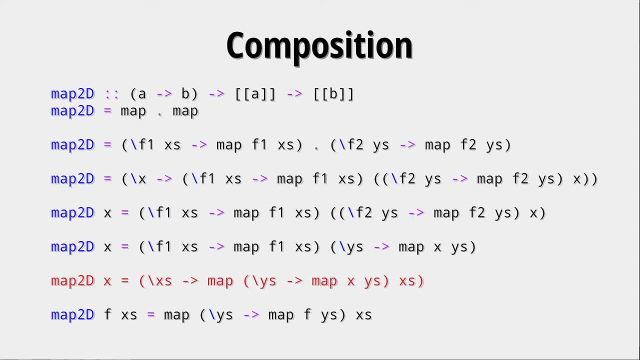 anonymous function. we have in the back ys mapped to xys. that is exactly that function. so now we can replace f1 with this anonymous function and after that we don't have to do much, because now we have the xs in the anonymous function here that we can take into the. 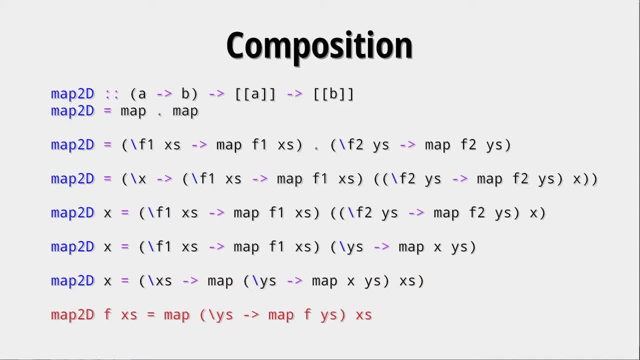 argument list of map2d. Now we rename x to f, because normally if you have a function within your, within your argument list, you would call it f or g or h, you wouldn't call it x. x is sort of a name you only give to elements of a list, for example, or something like that. But here now we 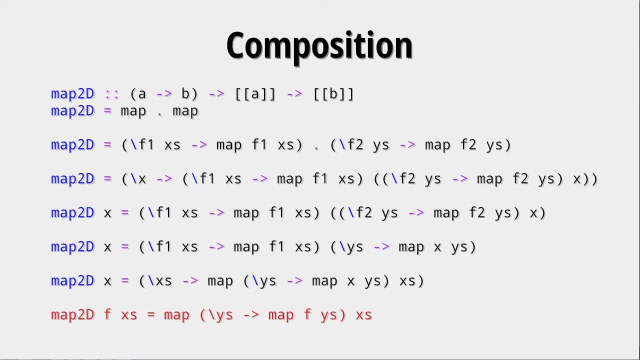 have a complete definition of map2d. well, we had a complete definition before, but now we sort of see this is a two-dimensional mapping. So here you have a function map2d that takes one argument, f, and an argument xs- f is a function and xs is a list- And then we do a mapping on this xs, where, for every 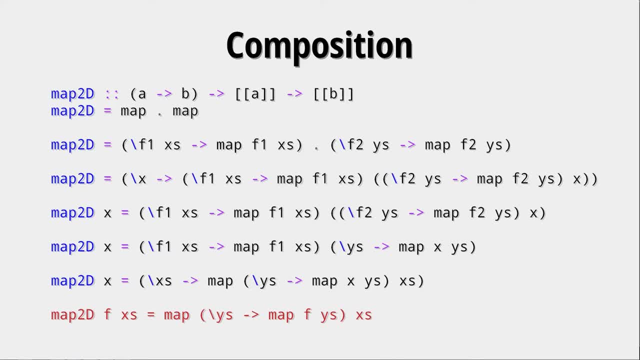 element, we do another mapping, Another mapping with this f function on the ys that we get within xs. f means that for this whole thing to work, xs has to be a list of lists. Okay, again, this also works with three-dimensional mapping and if you feel adventurous, you can try to do this sort of. 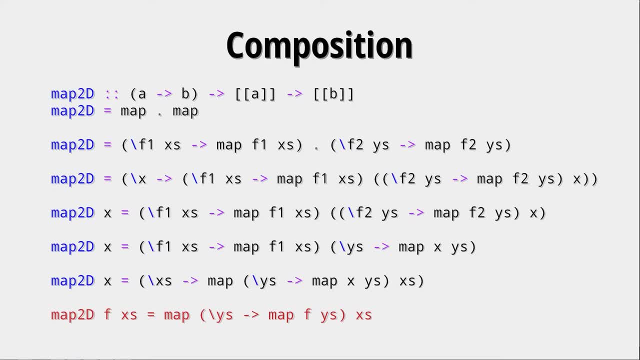 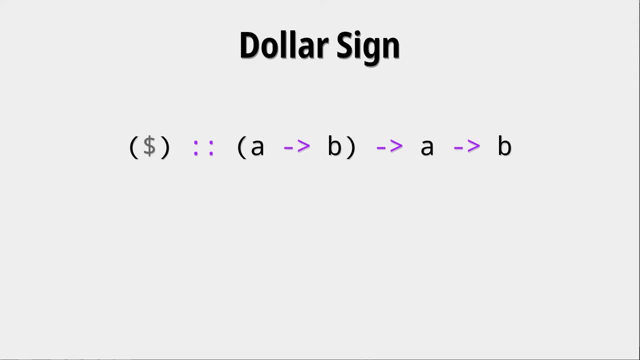 equivalency test on three-dimensional or even four-dimensional mappings. Another well, not that important but also somewhat important operator, which is not really used for composition but just for tidier syntax, is the dollar sign. It is basically the same function that we had right when we talked about higher order functions. There we had this app function. 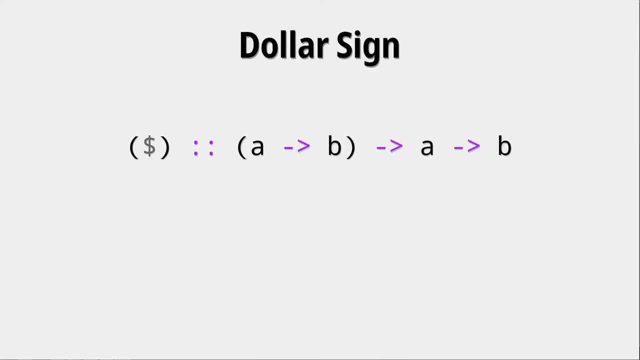 that took a function and its value and then just applied the function to the value. Well, that's exactly what the dollar sign sign is doing, but it can be written, and that's the important thing: it can be written In a cleaner and nicer way. Let's look at a very easy example for this dollar sign. So here we have. 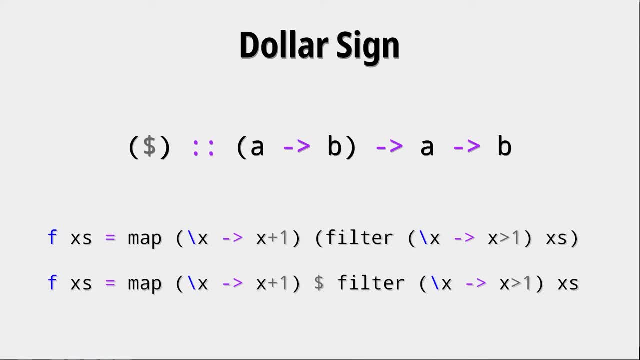 two definitions of some function. It's irrelevant what it does, but both definitions are the same. We see here that we have to put this term with the filter, the filter x axis greater, greater one xs. We have to put that in parentheses, otherwise this just wouldn't be correct. 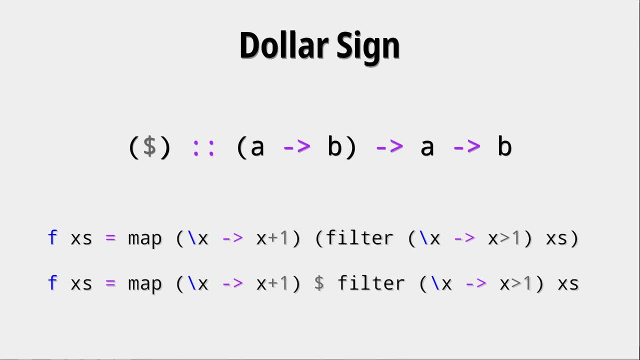 But sometimes we have to do this multiple times, where we have to write a lot of parentheses in order to get correct syntax. We don't have to do that when using the dollar sign, because now what we do here is say, well, we have this filter x to x greater than one, and we apply it to xs.